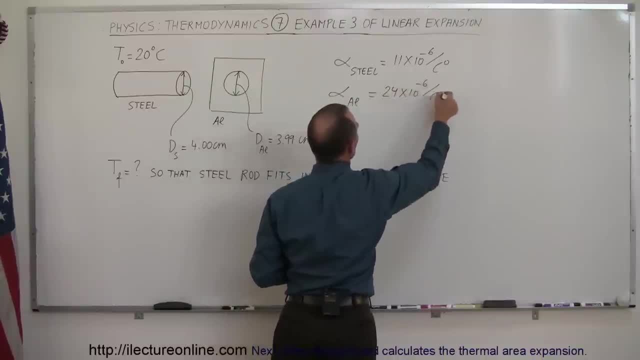 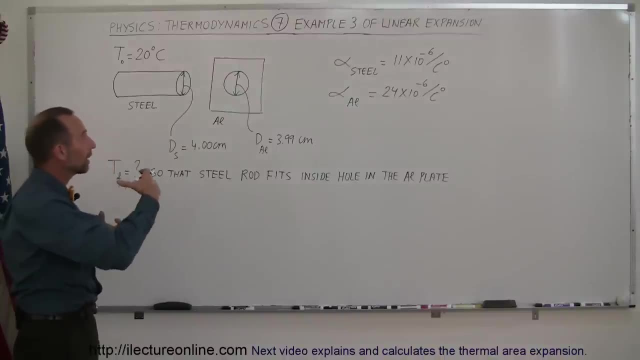 is equal to 24 times 10.. So you can see that the aluminum will expand more than the steel. That means the hole will get bigger faster than for steel, as they're being heated up to the same amount, the same temperature And eventually the steel rod will fit in there. Then, when you let that cool down again, of course the 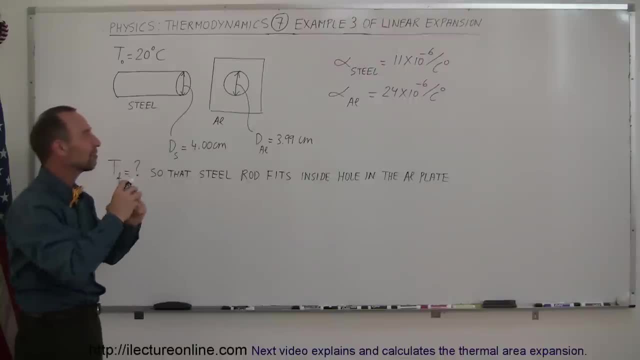 aluminum will then shrink more than the steel and make a very, very tight fitting around the rod, And the rod will not go anywhere after that. That's called heat fitting. That's still used in industry. So how high does the temperature need to be, And how high does the temperature need to? 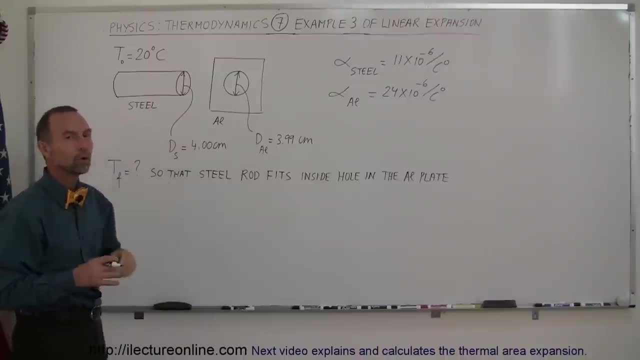 be for both metals, so that the rod will actually fit in the hole of the aluminum plate. And, by the way, something you may not realize is that, yes, when you heat up a plate that has a hole drilled in it, the hole will not get smaller with increasing temperature. The hole will actually get bigger with increasing 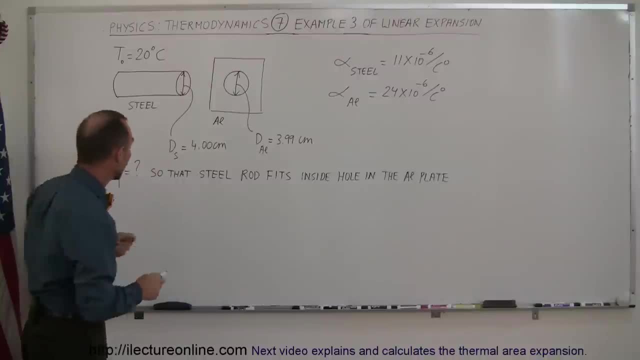 temperature, And we'll see later on another video why that is so. But now we're trying to figure out the final temperature. So how do we figure that out? Well, you see that the aluminum has to expand more than the steel. How much more, Of course, the difference between the aluminum and the steel. 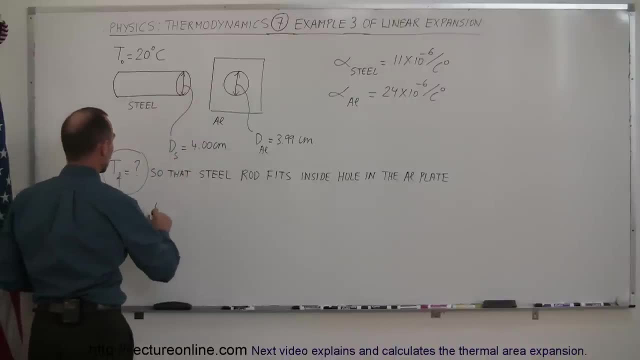 And so what you can say then is that the change of the aluminum in the length, the change in the length or diameter of the aluminum, is equal to the change of the steel. So let me put aluminum here, the change in the length of the steel plus 0.01 centimeters. That makes sense, right, Because the 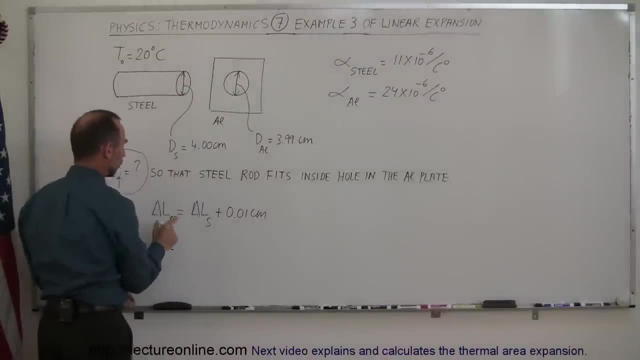 steel has to expand less than the aluminum, So the aluminum has to expand as much as the steel. plus this, so that the steel can fit. All right, That seems to make sense. Now let's plug in the equations. That means the coefficient of linear. 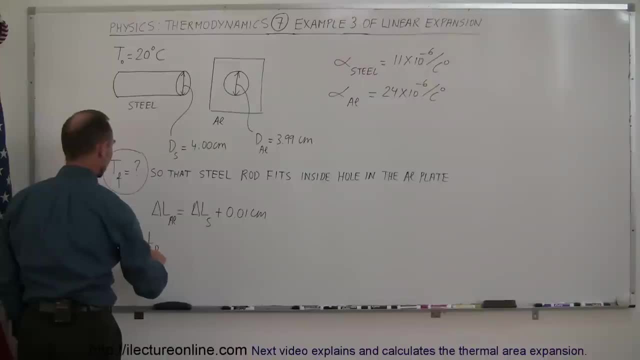 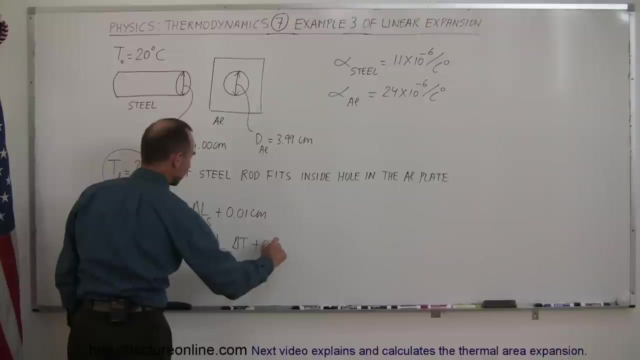 expansion for aluminum times, the original length of the aluminum times. the change in the temperature for the aluminum is equal to the linear coefficient for steel times. the initial length of the steel times, the change of the temperature for the steel plus 0.01 centimeters. And if I keep everything, 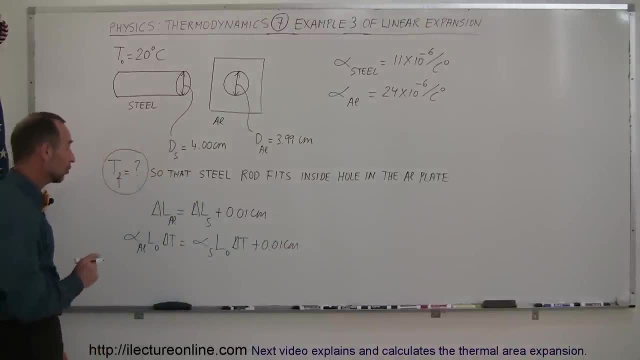 in terms of centimeters. I'm good with the units. Now notice that the change in the temperature for both is going to be exactly the same. So we can solve this equation for the change in temperature by first moving everything over to one side, So we could say that the change or the 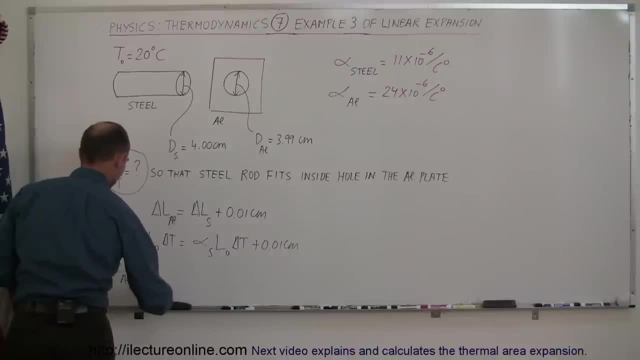 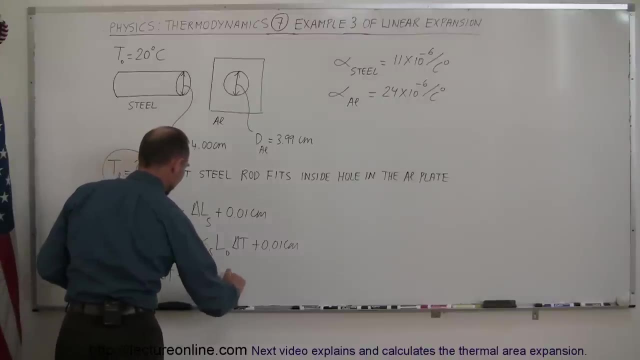 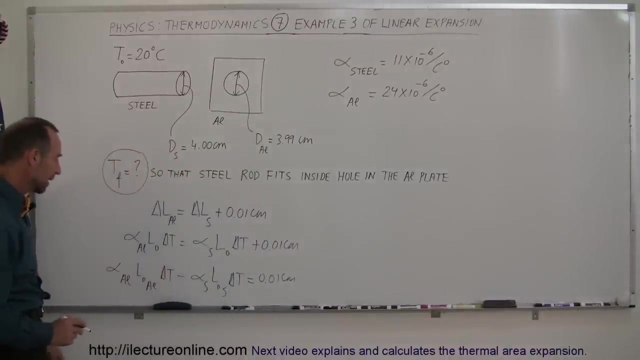 coefficient of linear expansion of aluminum times: the original length of the aluminum times, delta T, minus when we move this across the coefficient for steel times, the original length for steel times, delta T is equal to 0.01 centimeters. So now you can see that I can factor out a delta T and then 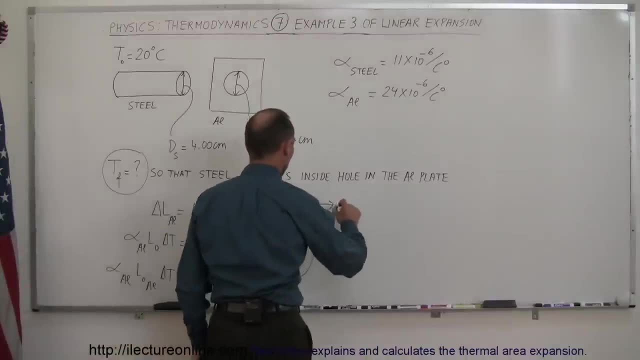 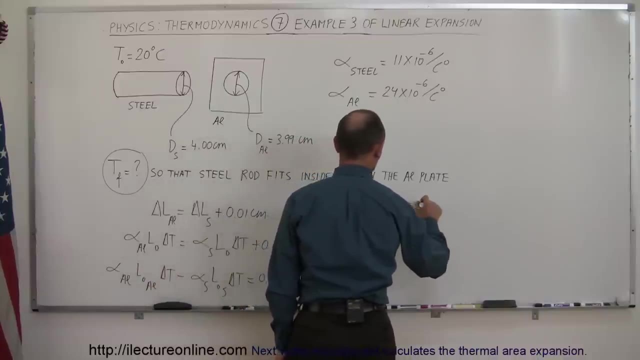 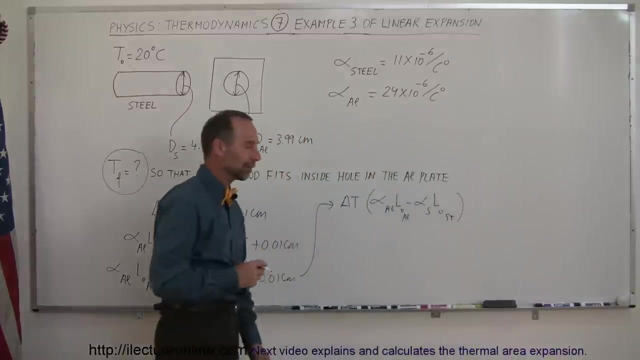 divide everything by what's left. So let's do that here. So I have delta T times what's left, which is the coefficient for aluminum times the original length for aluminum, minus the coefficient of steel times original length for steel. So I put aluminum here, steel there. I know I'm in your way, so let me get out. 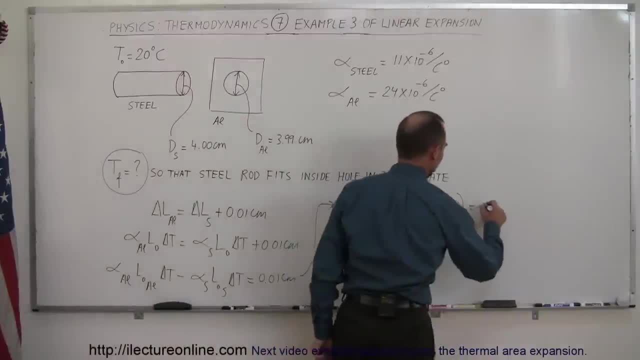 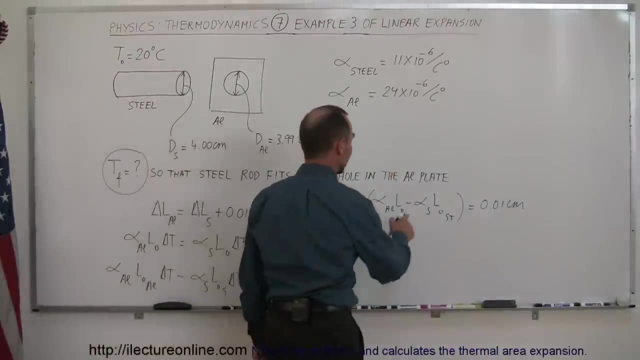 of the way here, so you can see that, And that then equals what we have on the right side, which is 0.01 centimeters. All right, Last thing we need to do is divide both sides by this, So we could say that the 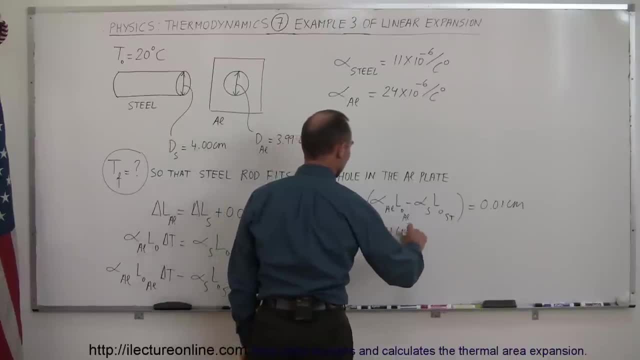 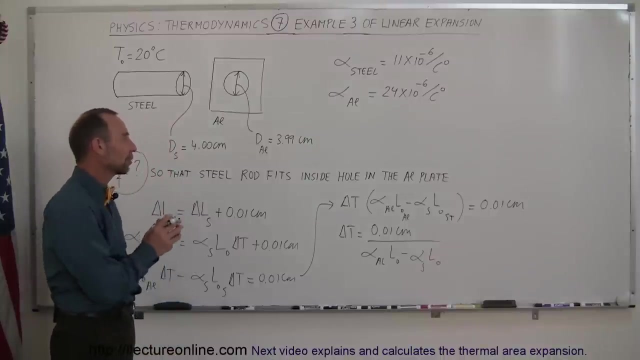 the temperature is equal to 0.01 centimeters divided by the coefficient for aluminum times original length minus the coefficient of steel times the original length. now you can probably be okay by saying that the original length for both is approximately the same. you can see that. 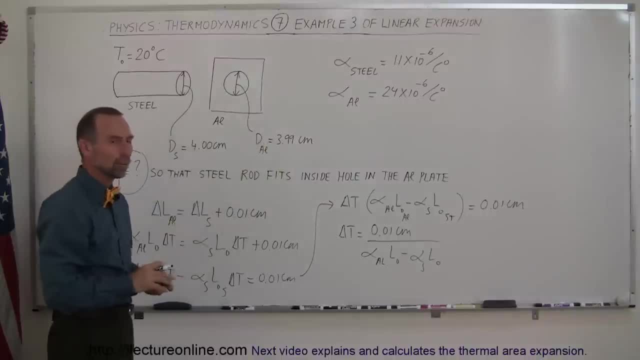 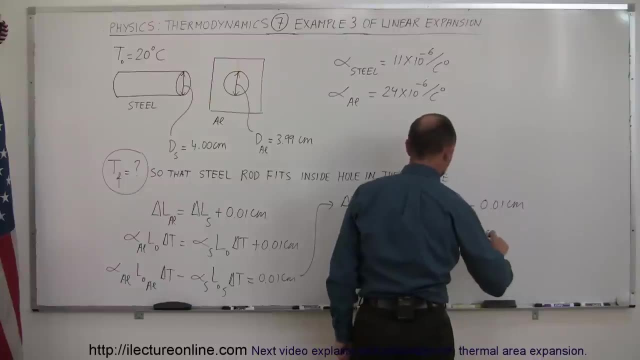 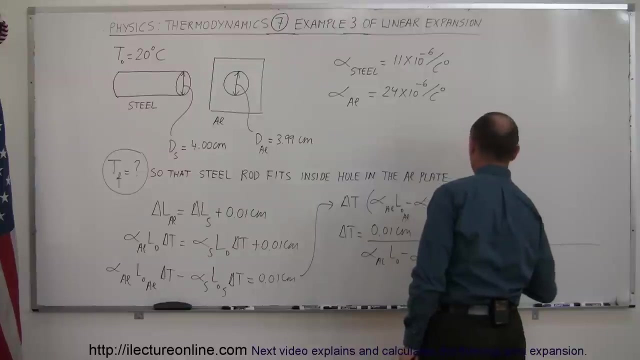 there's a very small difference between them, but just to kind of keep it exact, we'll go ahead and use the the proper numbers, all right? so this is equal to 0.01 centimeters divided by the coefficient of aluminum, which is 24 times 10, to the minus 6 percent of grade degree. 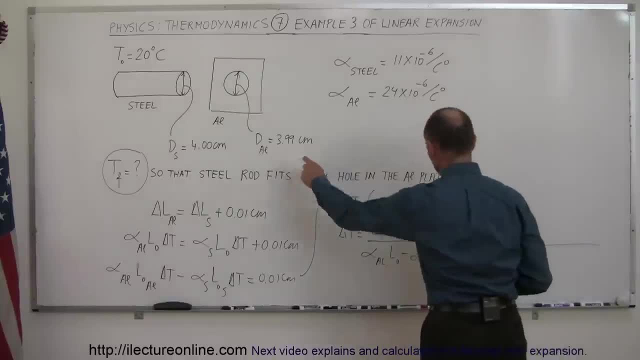 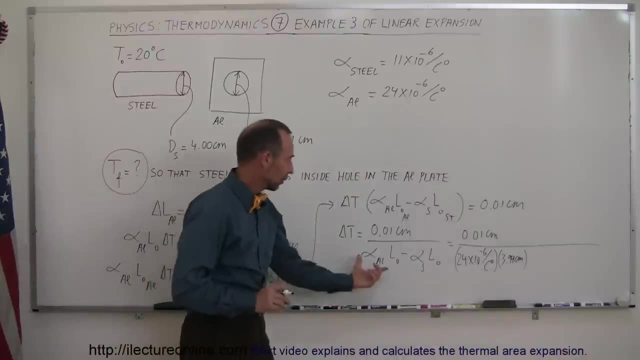 times l sub naught for aluminum, and for aluminum was 3.99 centimeters. so 3.99 centimeters- and let me get out of your way so you can see that right. so we just plugged in what these two are equal to. now we're going to plug in what these two are equal to. now we're going to plug in what these 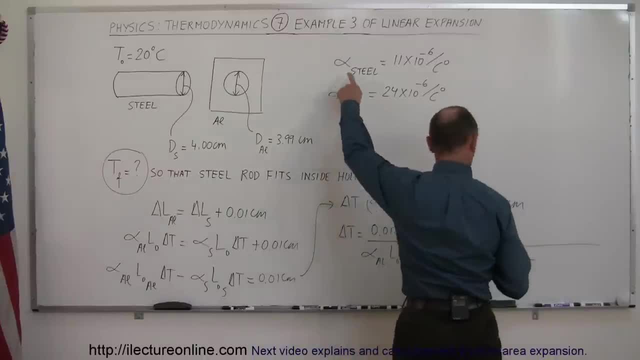 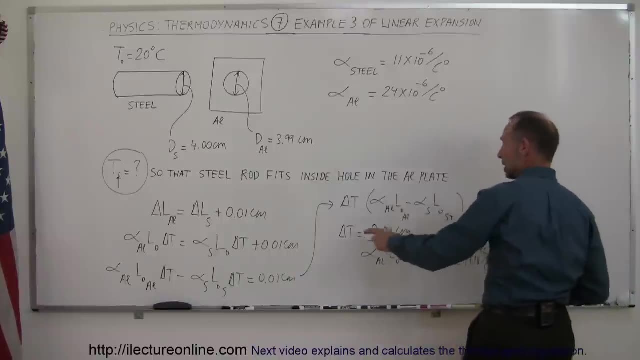 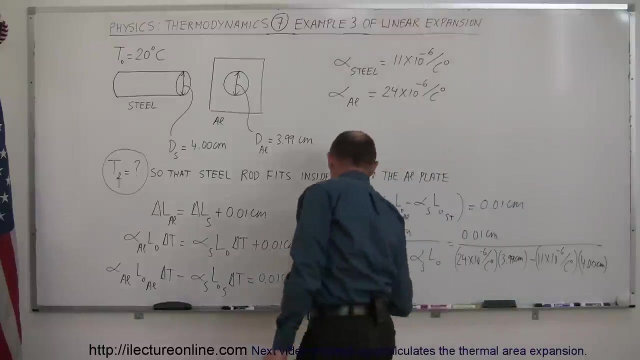 two are equal to now. we subtract from that for steel is 11 times 10 to the minus 6 percent of grade degree times, and that would be the exact diameter for steel, which would be 4.00 centimeters. all right, so this should give us the change in the temperature, and here's our calculator. 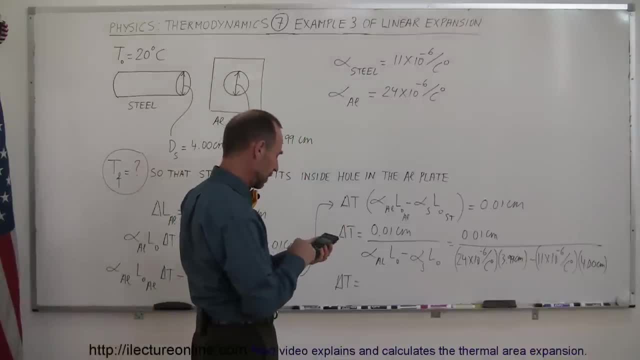 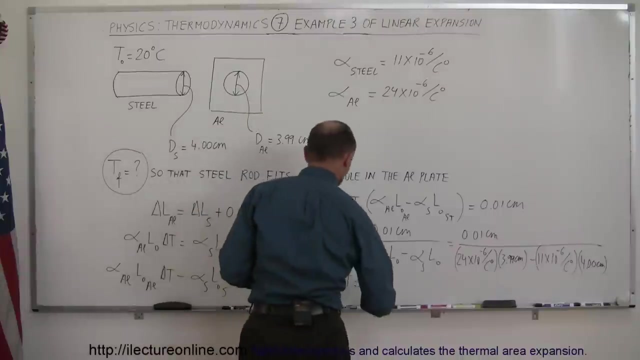 so let's first work out the denominator. so f 24 e, 6 minus times 3.99 minus 11 e to the 6 minus times 4 equals. take the inverse of that and then multiply the times 0.01 equals and i get 193 degrees- centigrade or centigrade degrees. so 193 centigrade degrees. 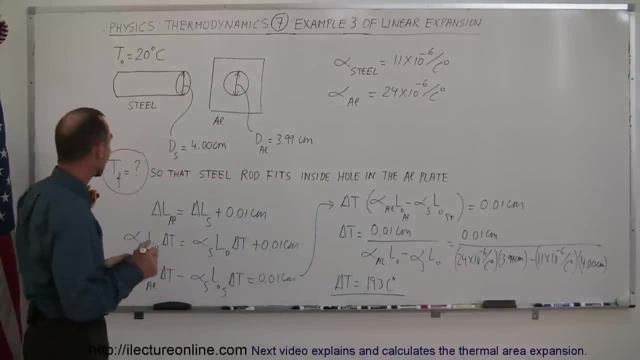 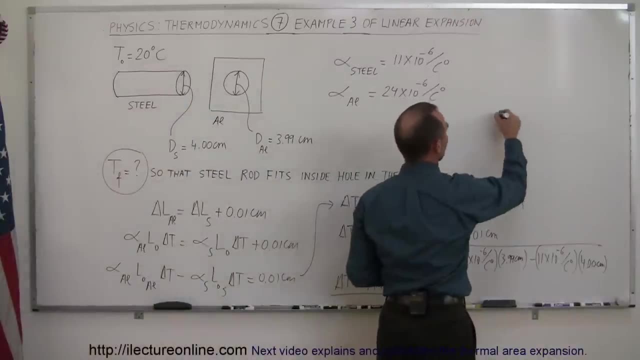 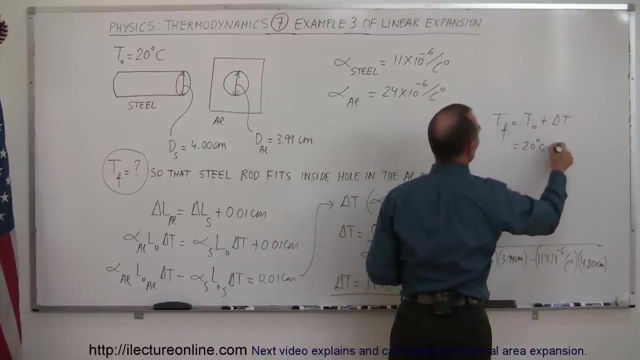 so if the increase has to be 193 centigrade degrees, the t final then must be this plus the t initial. so let's write that down here so we could say that t final is equal to t initial plus the change in the temperature. the initial temperature was 20 degrees centigrade plus a delta. 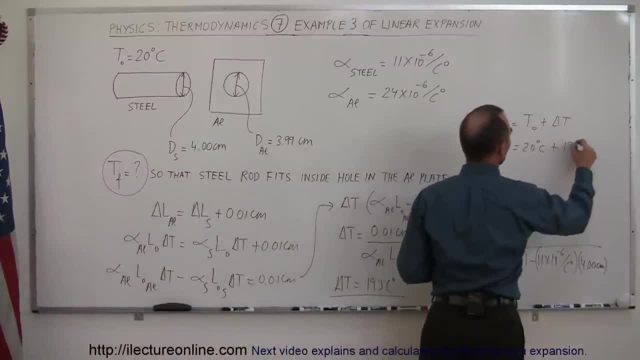 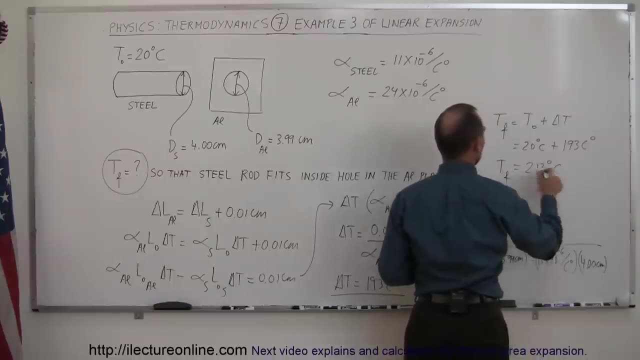 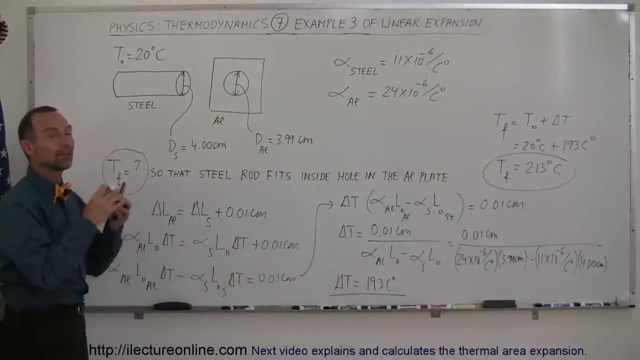 of 193 centigrade degrees- 193 centigrade degrees or so, that's equal to 213 degrees centigrade- for the final temperature. heat up to 213 degrees centigrade, then the steel rod will fit right in the hole. and then you, while you're heating up the steel row piece- the et favorite, just like all the 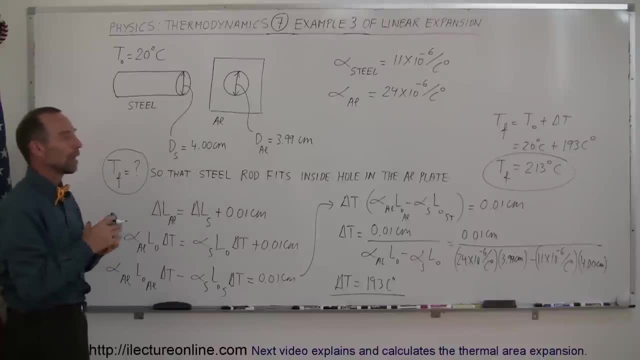 allow it to cool down and the aluminum will then clasp itself around the steel rod and you won't be able to move that rod anywhere. you probably want to heat it up a little bit more than that so it fits, because if you cut it that close you might have a little trouble getting the rod. 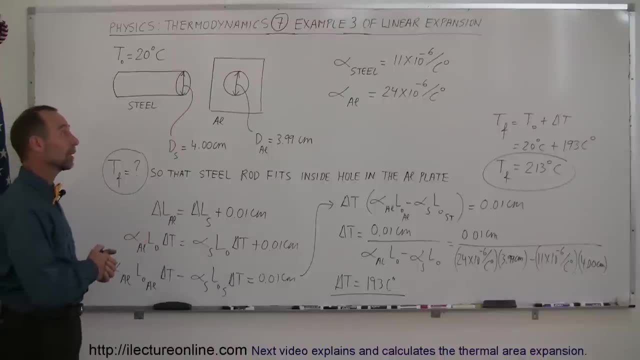 into the hole. anyway, that's a nice little example of how we work with linear expansion. 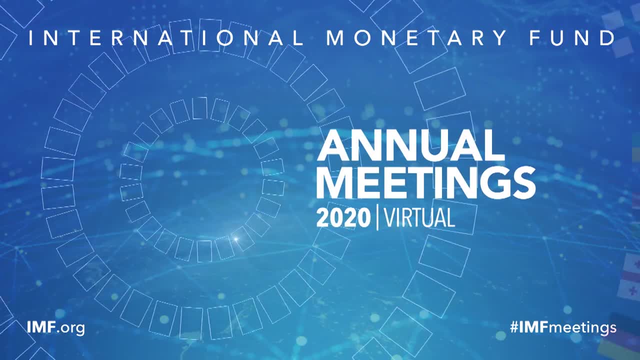 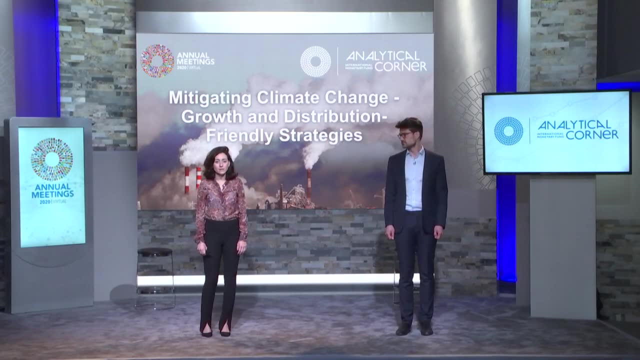 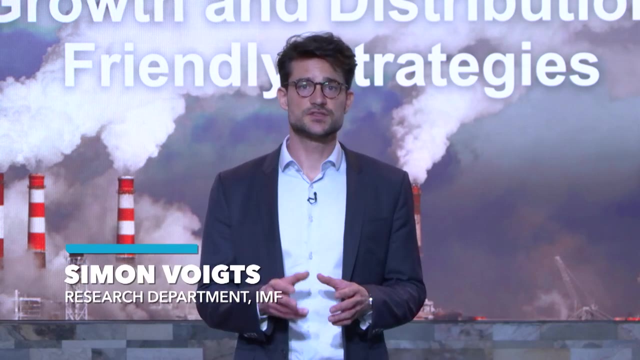 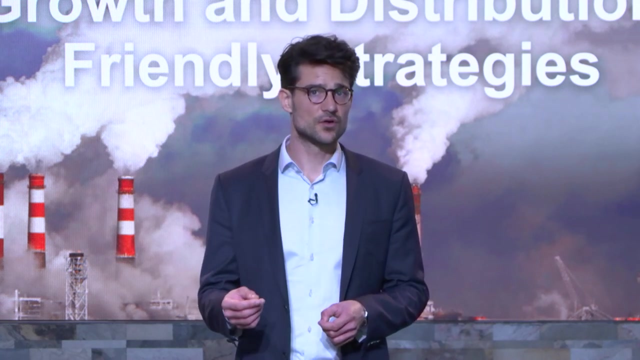 Welcome. I'm Simon Vogts And I am Marina Tavares, And we will present the climate change chapter in the World Economic Outlook. So what if I told you that when today's children are old, they will live in a world where one third of the global population has to migrate to another country, or even to another continent, because it has become too hot where they are living?